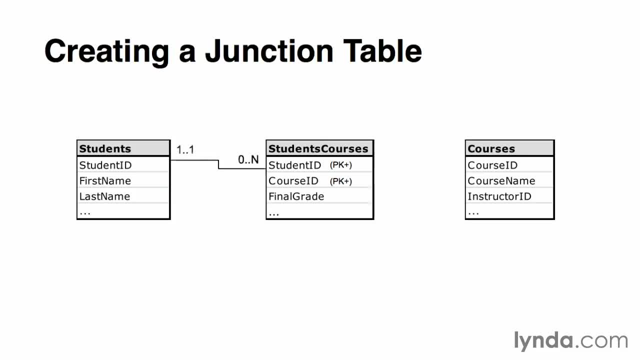 class. Each component of the key then gets related back to the original tables in a pair of one-to-many relationships. The student ID gets related back to the students table and the course ID gets related back to the courses table. Now we can create any additional fields in this linking table that further describe the. 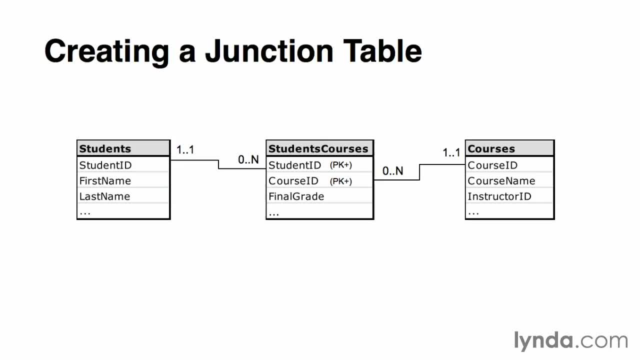 unique pairing of a student and a course. For instance, a final grade column is specifically about a student's performance in a single course. It's a perfect attribute to store in our new linking table, because it isn't really about just the student, It definitely isn't about just the course. 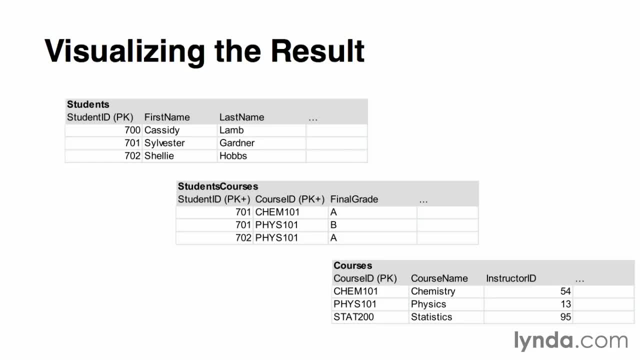 So the junction table will store a unique pairing of student ID and course ID in each record. Most students will appear lots of times, while brand new students won't appear at all in the linking table. The nice thing about this arrangement is that it doesn't prevent a student from being created. 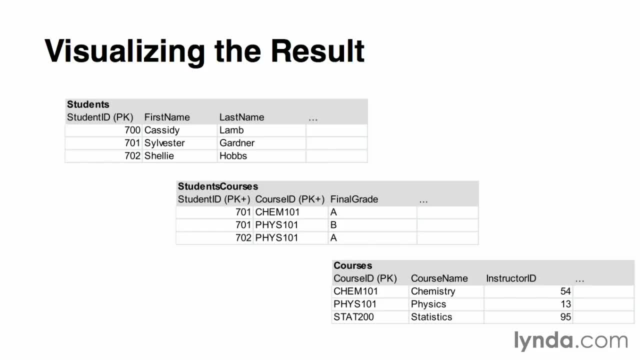 in the students table that hasn't yet registered for a class, And courses can be created in the course table even though nobody has yet registered. As soon as a freshman student registers for their first course, however, a new record in the linking table will appear. 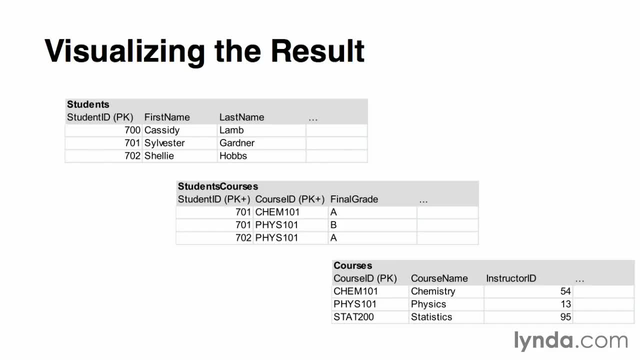 The link table will be created that identifies their student ID and the course ID they registered for. Now, as we read the diagram, we can easily identify all of the courses that a particular student has taken and easily get a roster of students registered for a particular course. 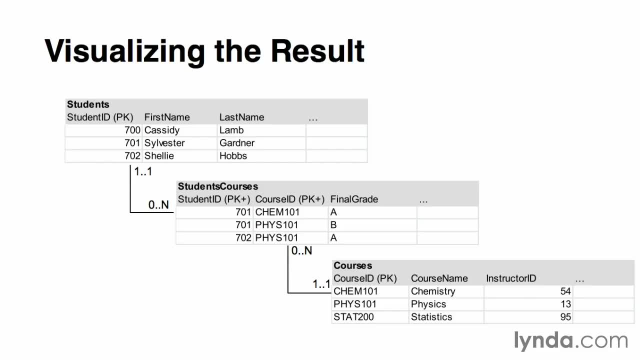 This is how a many-to-many relationship gets represented in the DBMS. In reality, they become a pair of one-to-many relationships that pass through this intermediary junction table. In preparation for moving our design into the production phase, we need to accurately resolve all of our many-to-many relationships. 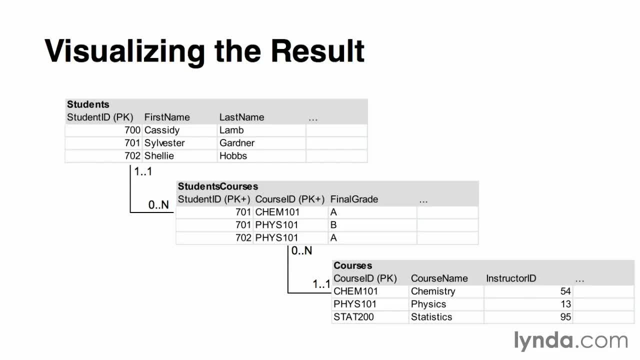 To do this, you'll print out a new table design worksheet for each many-to-many relationship in your data model. give the new table a suitable name and fill in the names and data types for the composite key columns by copying the name and data type from the two original tables. 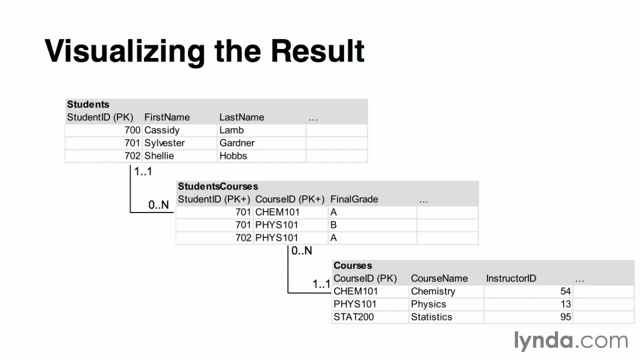 Finally, think through your original business rules and interview sessions to determine whether there is any additional information that is uniquely captured by this intersection of values, and add them back into your data model diagram. This is how a many-to-many relationship looks like in the DBMS. Subtitles by the Amaraorg community.